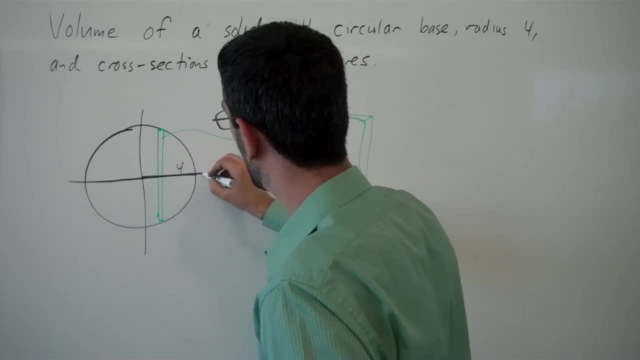 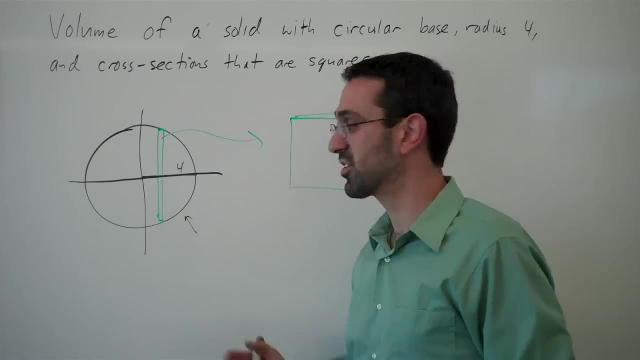 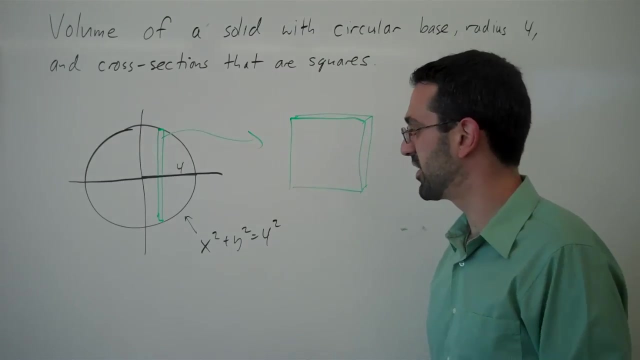 So to do that first thing we're going to do is introduce a coordinate system here so that we have an origin there to work with and then we can write an equation for this circle. So x squared, So x squared plus y squared equals radius squared gives me an equation for that, for that circle. 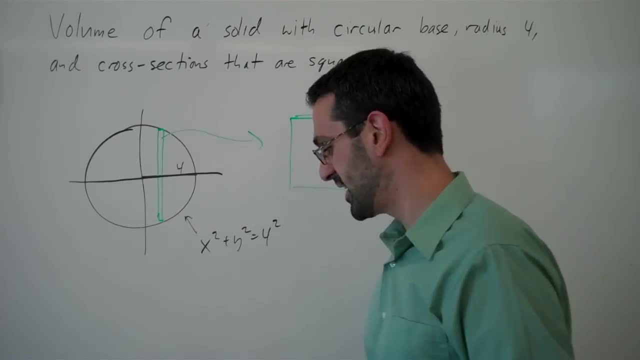 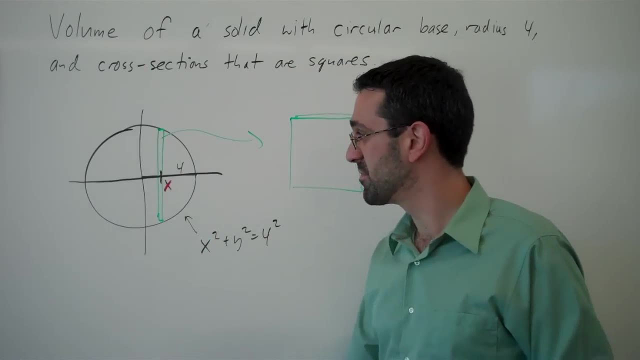 Next, I need to introduce a variable for where I am slicing, And here it looks like the x value is giving me the location of the slice. So now, from that x value, I need to know how tall my slice is. 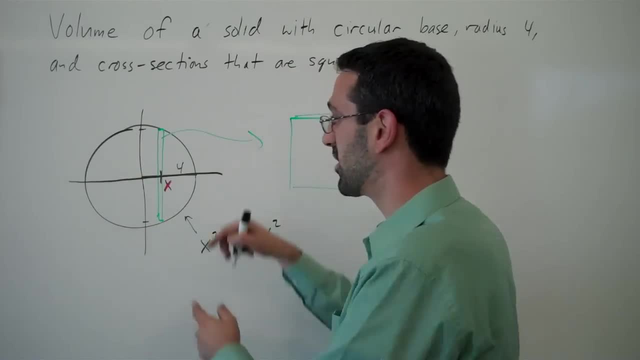 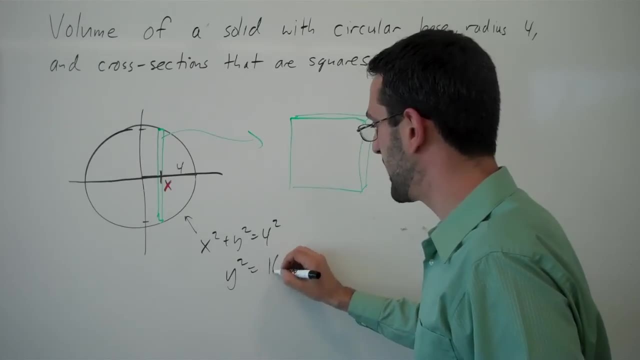 So for that I need to know what these y values are So I can find the height, So solving my equation here: y squared equals. let's go ahead and square that: 16 minus x squared, y is plus or minus root: 16 minus x squared. 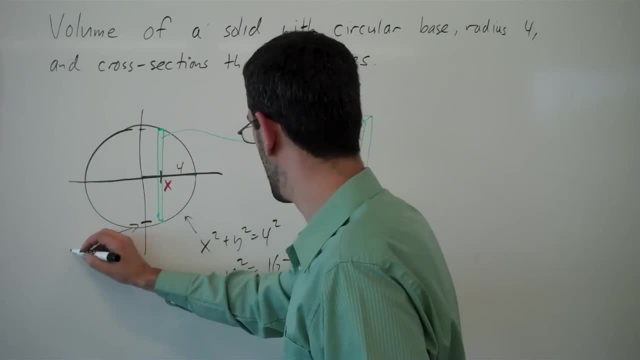 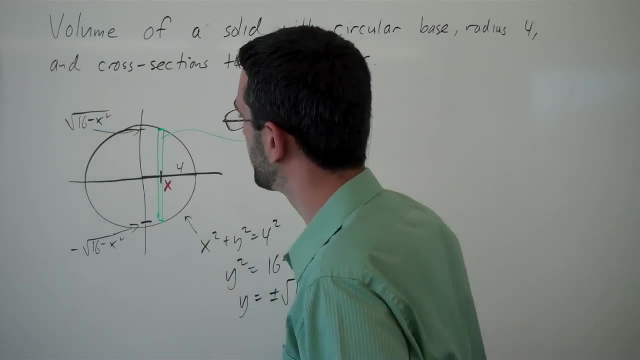 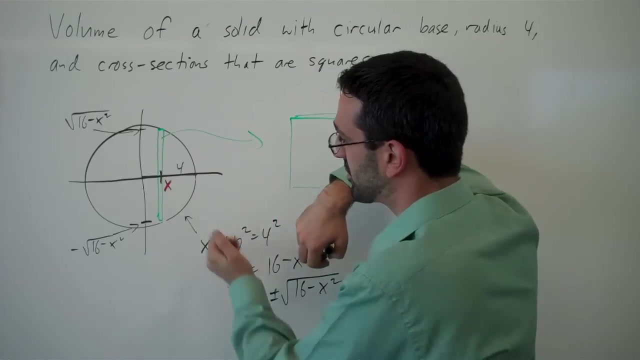 And so my y value here is the negative square root and the y value here is the positive square root, right, And the total height then is the difference between those. Or you could also think of it as this height is root 16 minus x squared. this is the same. 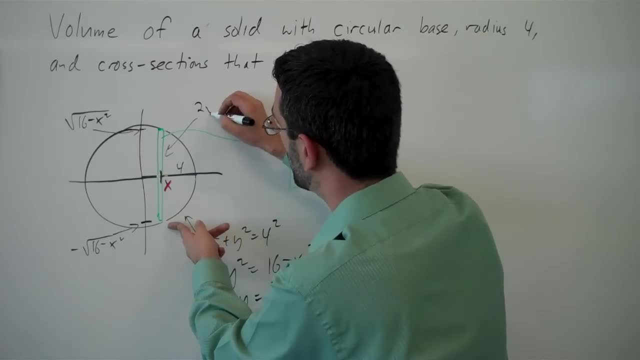 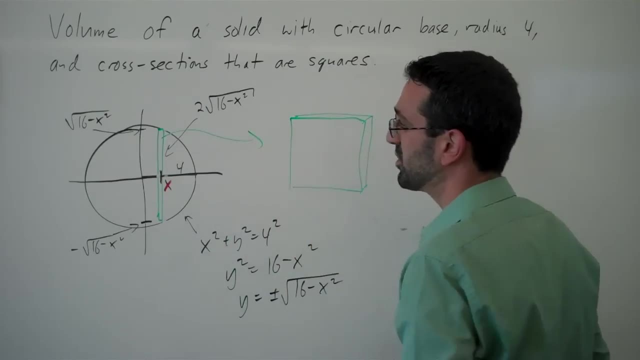 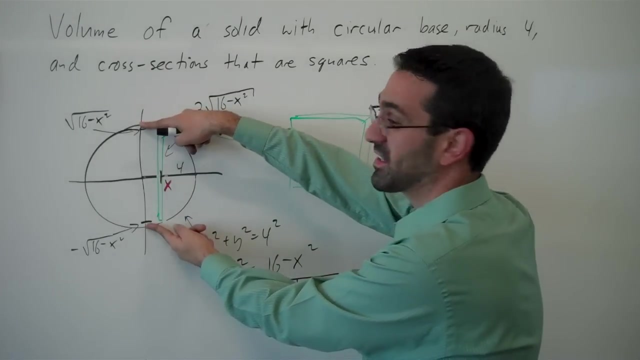 And so this entire height will be 2 square root of 16 minus x squared. Okay, Notice that this works the way we would expect. When x is 0, then this value is going to be very large. We're going to have a total height of 8.. 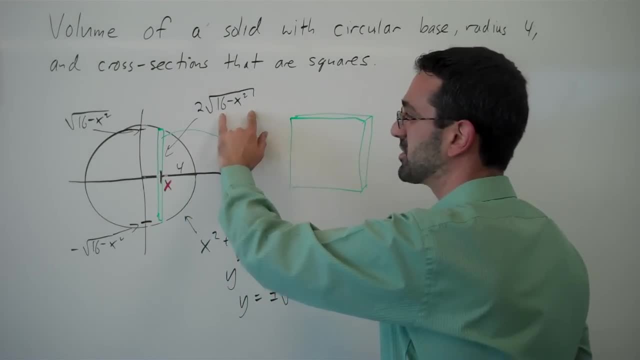 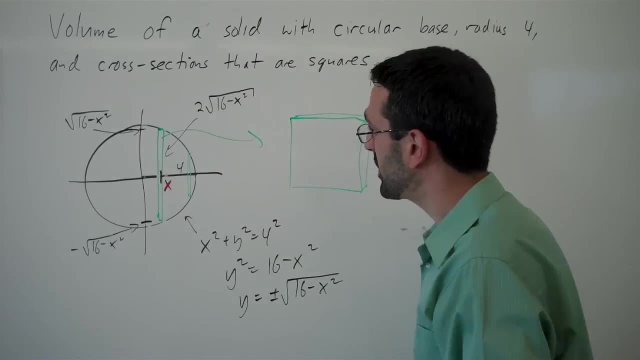 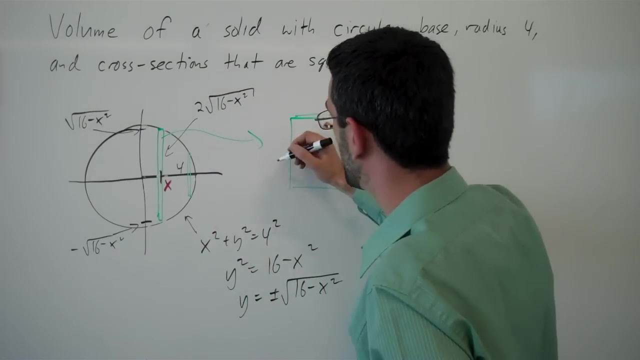 When x gets close to 4, then this value is going to get much smaller Because the slices over here are going to be much shorter. So the length of this side corresponds with this side of my slice. So this is 2 root 16 minus x squared. 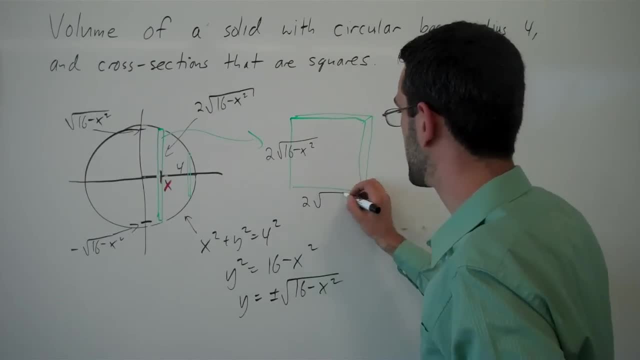 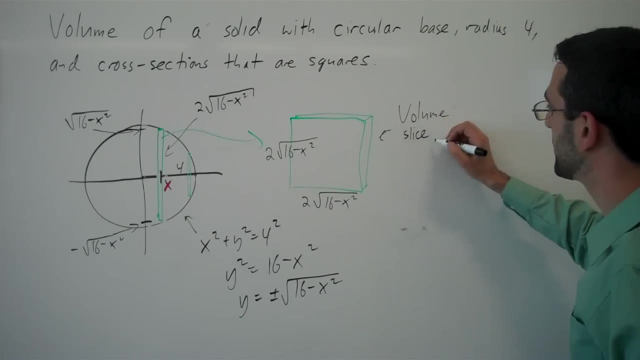 And because it's a square, this side has the same length. So now we can write an equation for the volume of this slice. So it's A rectangular solid. we have length 2 times root, 16 minus x squared.